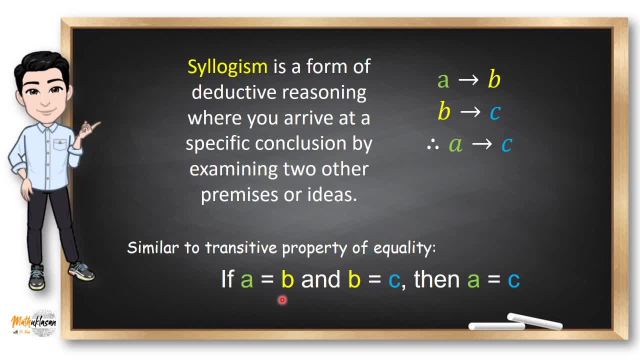 where, if we have A plus B or A equals B as our premise and B equals C as another premise, then A equals C because both are equal to B. Deductive reasoning is the drawing of inferences or conclusions from known or assumed facts. For example, all men are mortal. 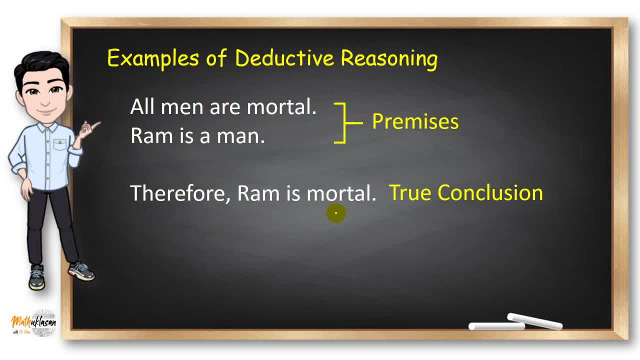 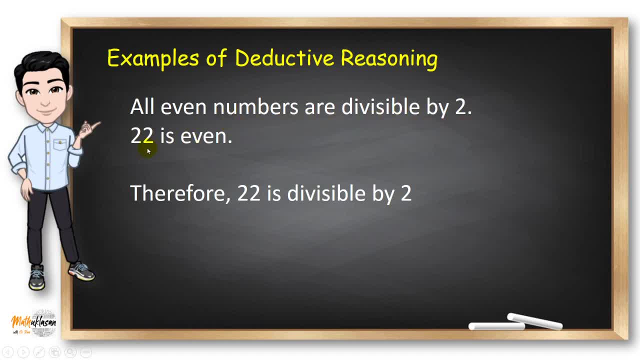 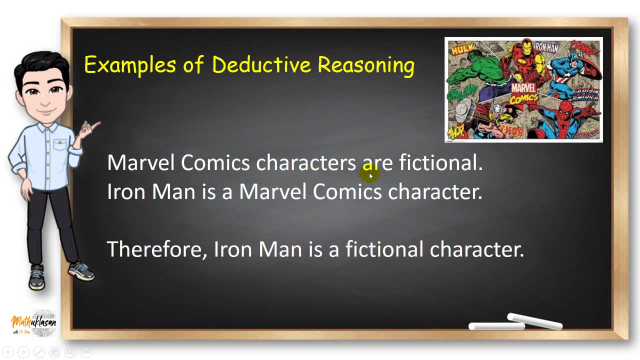 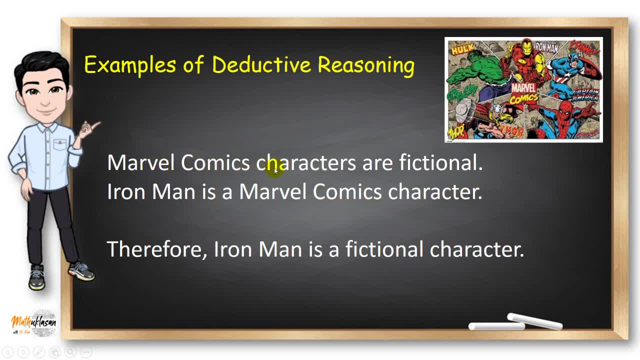 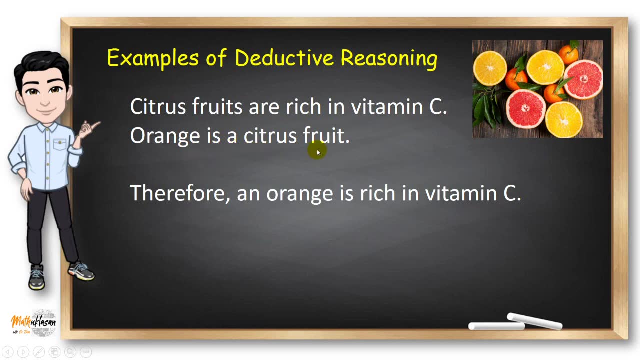 So we have here comics character as the same idea. So therefore, Iron Man is a fictional character Or is it dealing with a History of the Universe character? Let us see what you have here. Sitrus fruits are rich in Vitamin C. Orange is a citrus fruit. 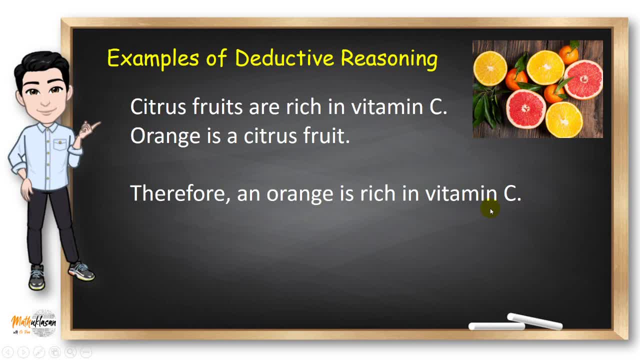 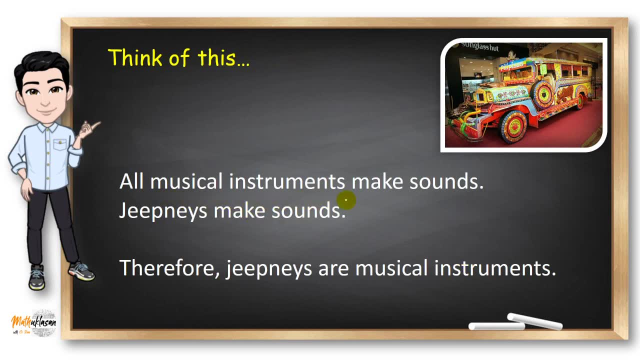 Therefore, orange is rich in Vitamin C. Now how about this example: All musical instruments make sounds. Jeepneys make sounds. Therefore, Jeepneys are musical instruments. Wait, wait, wait. All musical instruments make sounds. This is true. This is a true premise. 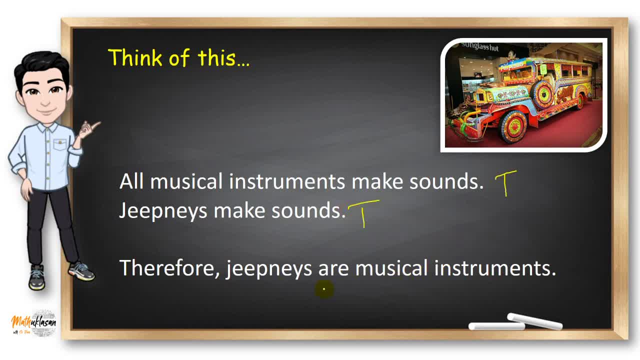 Jeepneys make sounds. This is also a true premise, But jeepneys are not musical instruments, so this is false. Therefore, this is not a valid deductive reasoning. Always remember that we use premises to prove the conclusion is true and not to justify it. 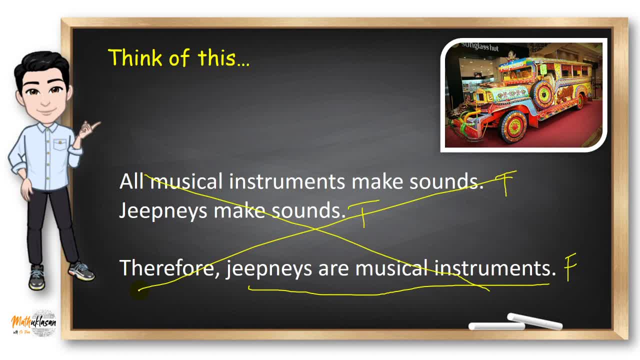 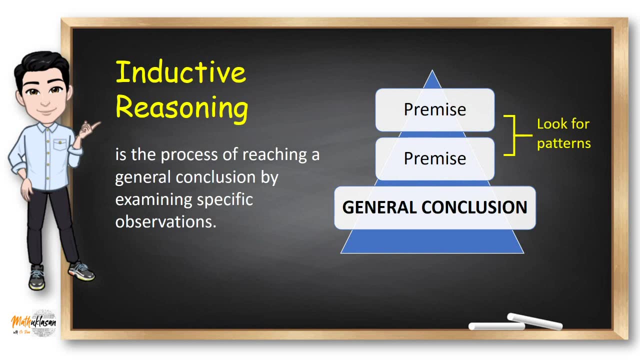 Deductive reasoning is meant to demonstrate that the conclusion is absolutely true based on the logic of the premises. Inductive reasoning, on the other hand, is the process of reaching a general conclusion by examining specific observations. So a few particular premises create a pattern which gives way to a general conclusion that is likely true. 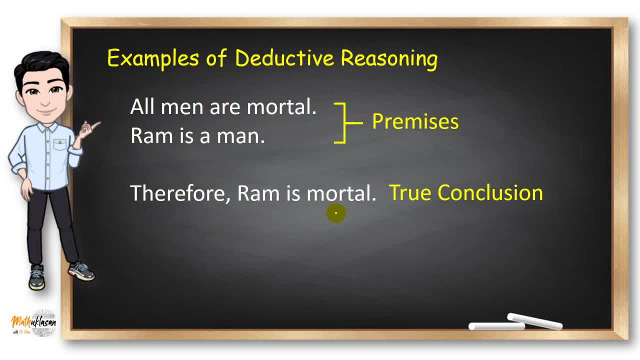 Ram is a man, therefore Ram is mortal. In symbols let this B implies C And this one B. A implies B, So we can see here that B are the same, So A implies C. Another example, Another example. 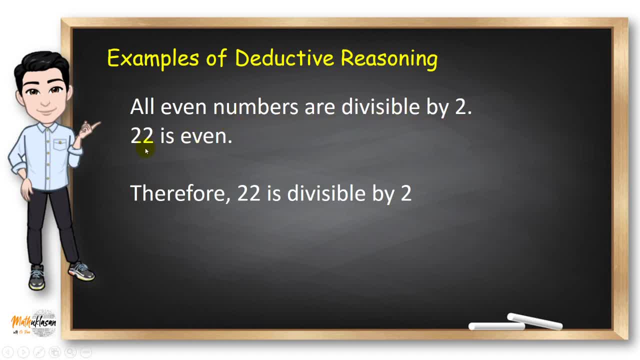 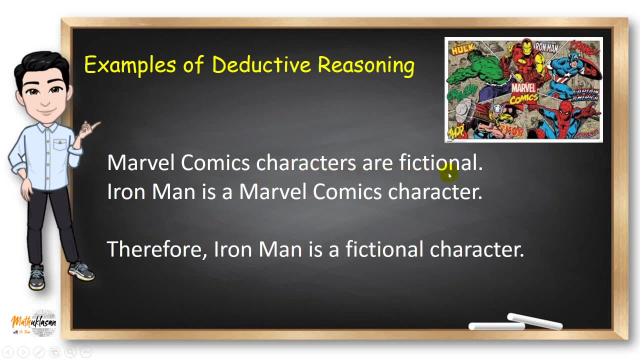 All even numbers are divisible by 2.. 22 is even, Since we have the same idea here. therefore, 22 is divisible by 2.. Next, Marvel Comics characters are fictional. Iron Man is a Marvel Comics character, So we have here comics character as the same idea. 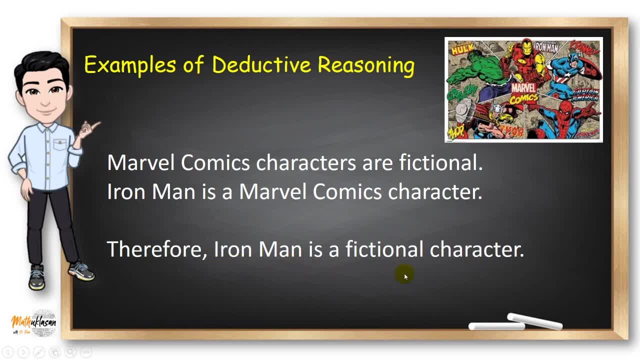 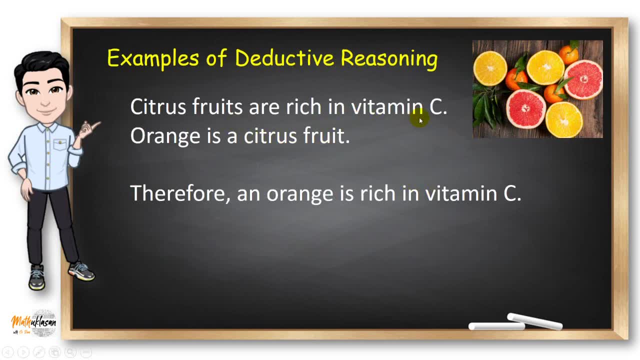 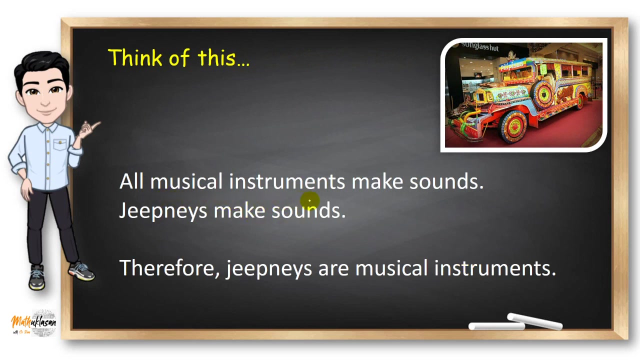 So, therefore, Iron Man is a fictional character. This is how we have to name this character. citrus fruits are rich in vitamin C. orange is a citrus fruit. therefore, an orange is rich in vitamin C. now, how about this example? all musical instruments make sounds. jeepneys make sounds. therefore, jeepneys are musical. 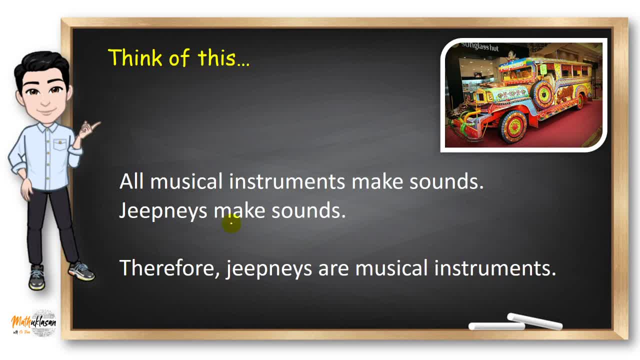 instruments. teka, teka, teka. all musical instruments make sounds. this is true. this is a true premise. jeepneys make sounds- this is also a true premise- but jeepneys are not musical instruments, so this is false. therefore, this is not a valid deductive reasoning. always remember that we use premises to prove. 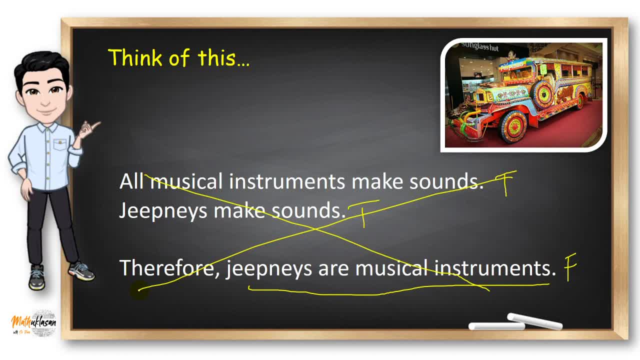 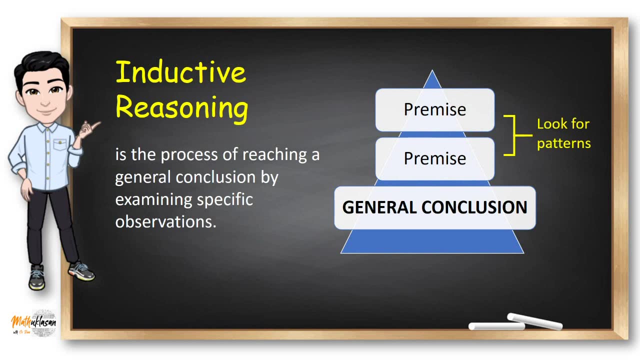 the conclusion is true and not to justify it. deductive reasoning is meant to demonstrate that the conclusion is absolutely true based on the logic of the premises. inductive reasoning, on the other hand, is the process of reaching a general conclusion by examining specific observations. so a few particular. 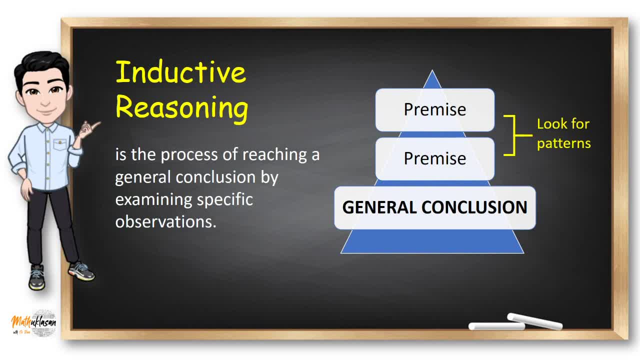 premises create a pattern which gives way to a general conclusion. that is likely true. this is commonly shown using a triangle that starts at the narrow premises and expands into a broader conclusion. unlike deductive reasoning, inductive reasoning has no basic standard format when we use it, so as long as we are finding a 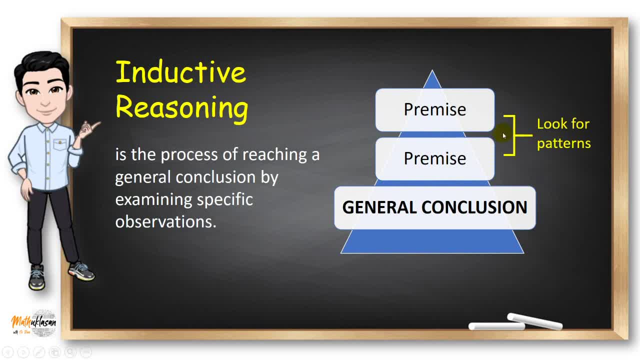 This is commonly shown using a triangle. A triangle is a window that starts at the narrow premises and expands into a broader conclusion. Unlike deductive reasoning, inductive reasoning has no basic standard format when we use it, So as long as we are finding a conclusion that is most likely to fit the premises, 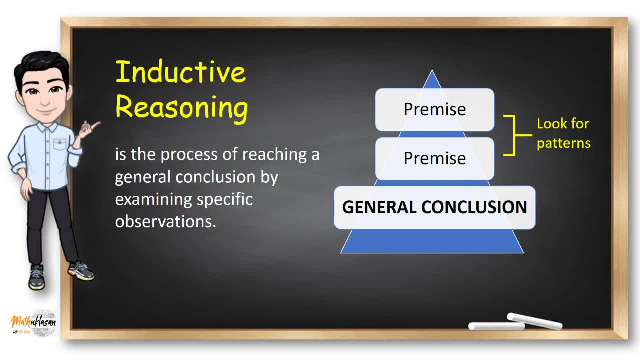 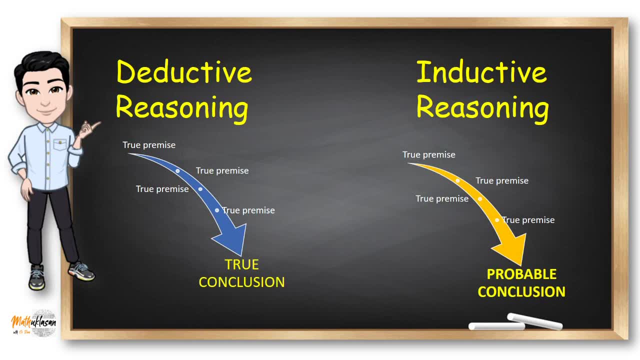 then we can make predictions, create generalization and analyze cost and effect. Keep in mind that in deductive reasoning, premises are used to prove a conclusion, While premises in inductive reasoning are used to predict a conclusion, Meaning we don't create a definite answer, but we are trying to show that the conclusion is the most probable one given the premises. 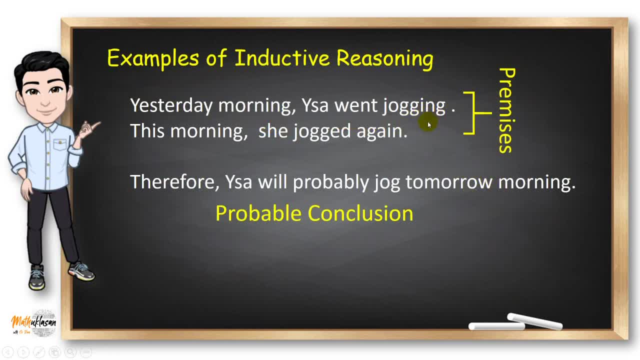 For example, yesterday morning Isa went jogging. This morning she jogged again. Therefore, Isa will probably jog tomorrow morning. This conclusion is not definite. Based on the morning routine of Isa, there is a high chance that she will jog tomorrow morning, right? 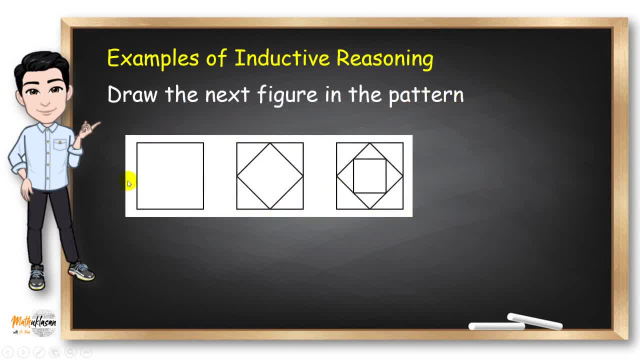 Now what if we are asked to find the next figure in this pattern? The first figure is a square. In the second figure, a second square was constructed inside of the first square, wherein the vertices of this new square are on the midpoints of the sides of the first square. 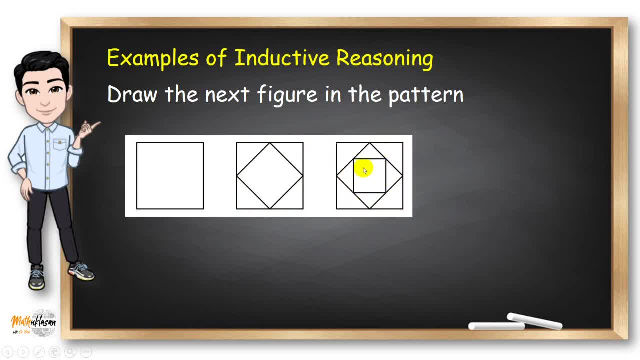 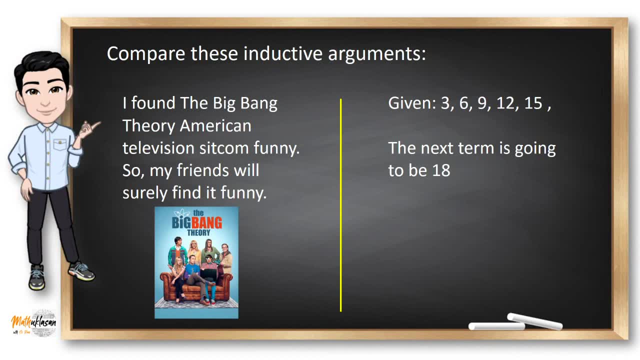 Following the same pattern and by using inductive reasoning, it's possible that the next pattern is this one: An inductive argument is either considered weak or strong based on whether its conclusion is a probable explanation for the premises. Let's compare these inductive arguments. 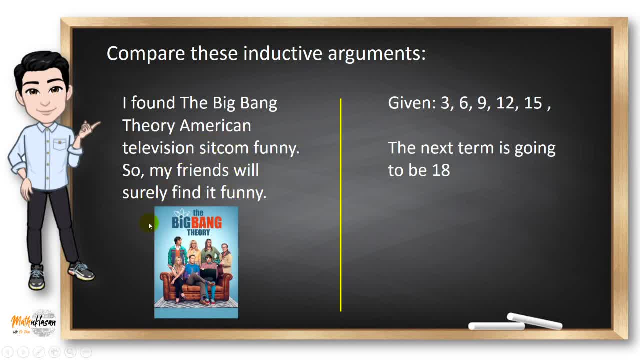 On the left. the two statements are likely true on their own, but the first premise does not predict the second to be true, Because I probably know what's funny for my friends, but some may find it corny. right On the right, we can see that these numbers are all multiples of 3, in ascending order. 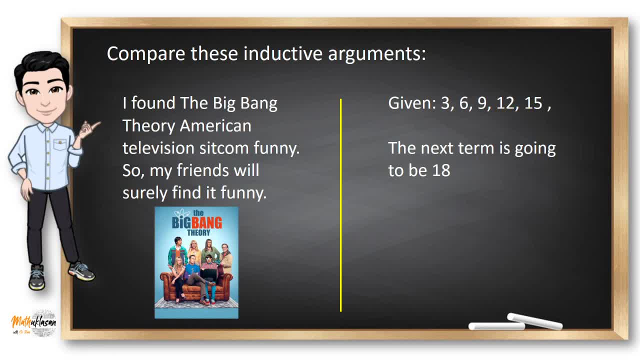 So it is logical to say that the next term after 15 is 18, because the premises identify a pattern. Thus the reasoning on the left is weak. Thus the reasoning on the left is weak while the right is strong. 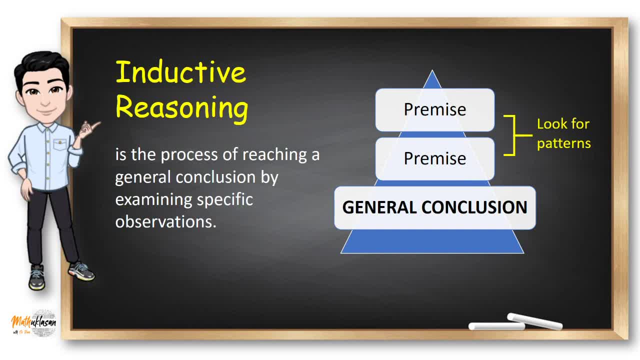 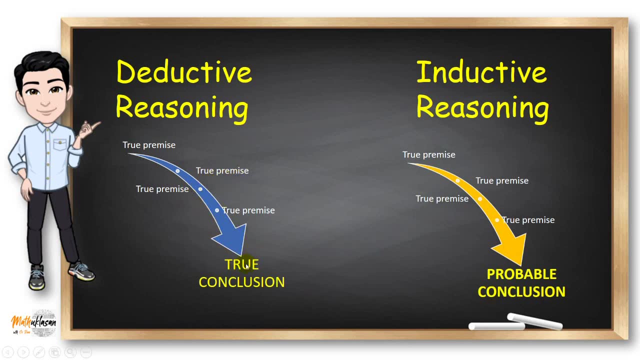 conclusion that is most likely to fit the premises. then we can make predictions, create generalization and analyze cost and effect. keep in mind that in deductive reasoning premises are used to prove a conclusion, while premises in inductive reasoning are used to predict a conclusion, meaning we 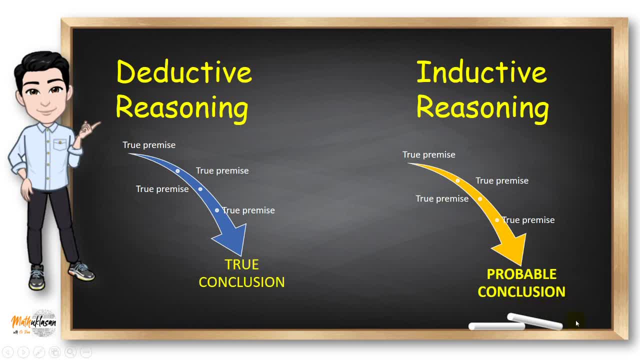 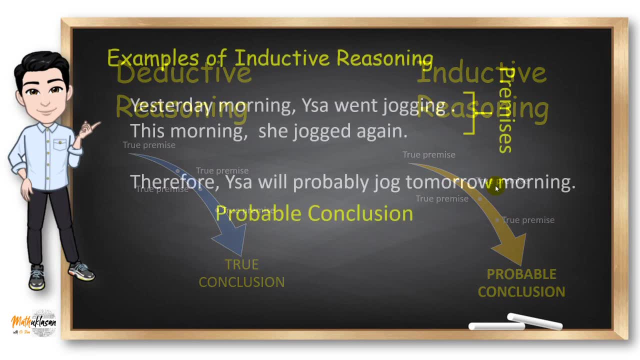 don't create a definite answer, but we are trying to show that the conclusion is the most probable one given the premises. for example, yesterday morning Isa went jogging. this morning she jogged again. therefore Isa will probably jog tomorrow morning. this conclusion is not definite but basing on the morning routine, 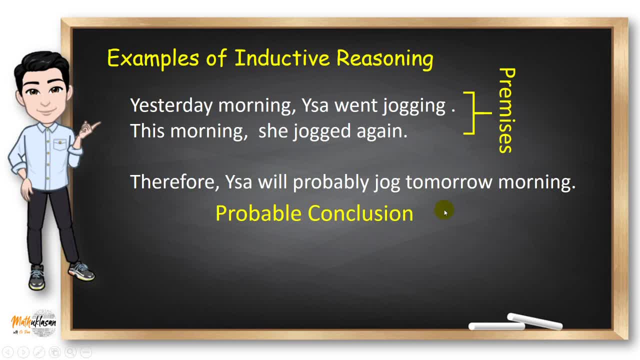 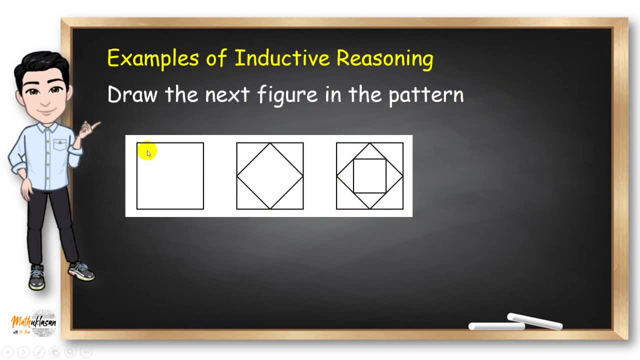 of Isa. there is a high chance that she will jog tomorrow morning right now. what if we are asked to find the next figure in this pattern? the first figure is a square. in the second figure, a second square was constructed inside of the first square, wherein the vertices of this new square are on the midpoints of. 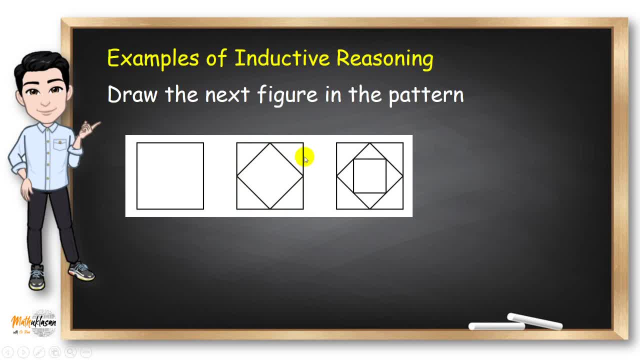 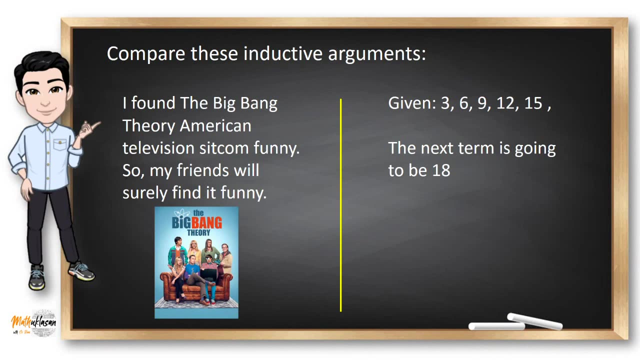 the sides of the first square following the square. this is the existing pattern and by using inductive reasoning, it's possible that the next pattern is this one. an inductive argument is either considered weak or strong based on whether its conclusion is a probable explanation for the premises. let's compare these inductive arguments on the. 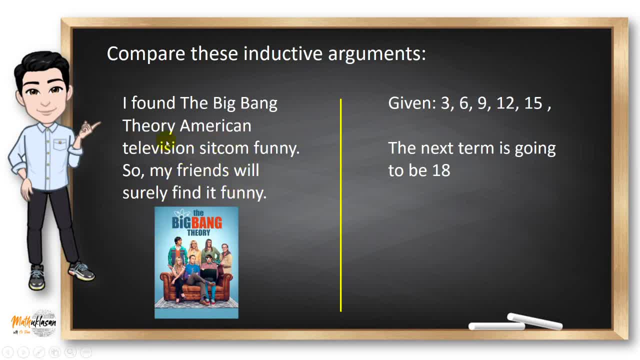 left. the two statements are likely to on their own, but the first premise does not predict the second to be true, Because I probably know which one is true. know what's funny for my friends, but some may find it corny. right on the right we can see that these numbers are all multiples of three in ascending. 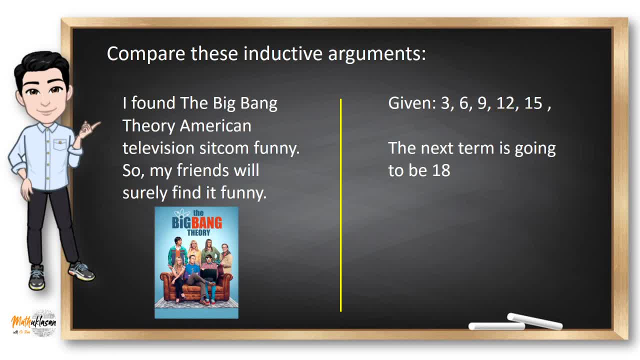 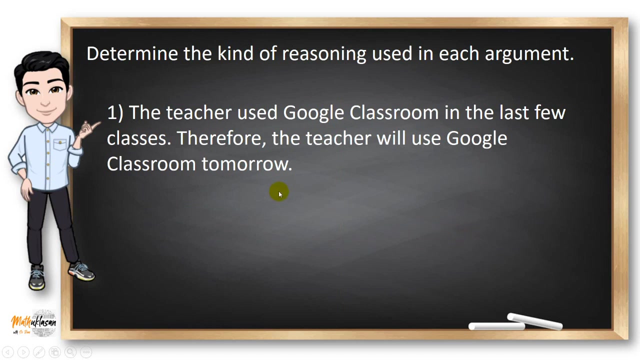 order. so it is logical to say that the next term after 15 is 18, because the premises identify a pattern. thus the reasoning on the left is weak, while the right is strong. now let's try determining the kind of reasoning used in each argument. for number one, the teacher used Google classroom. in the